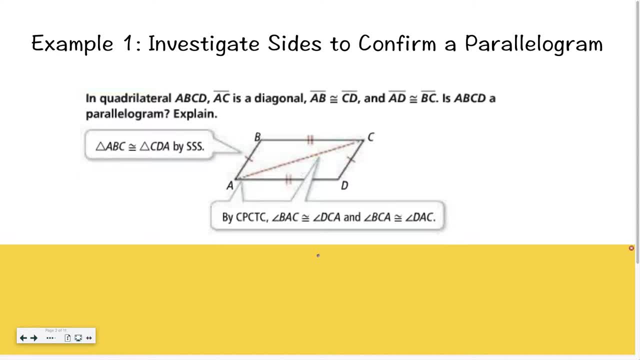 and we know that segment AB is congruent to segment CD and segment AD is congruent to segment BC. so you can see all of those markings are drawn in. there is ABCD, a parallelogram explained. So here we know that. 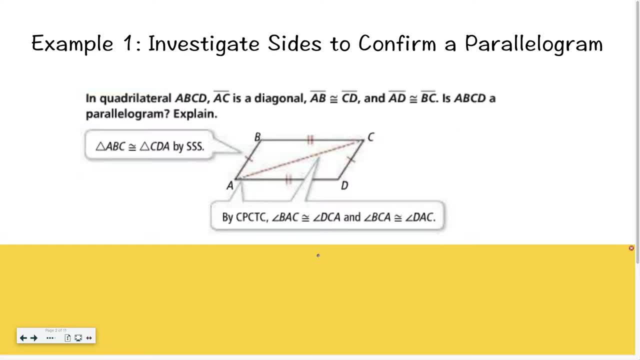 all of the sides are the same. right We have AB is congruent to CD. so these two blue sides are congruent to each other. We have these two purple sides are congruent to each other. and then we know that the dashed line, the diagonal down the middle, would be congruent to itself on both triangles. 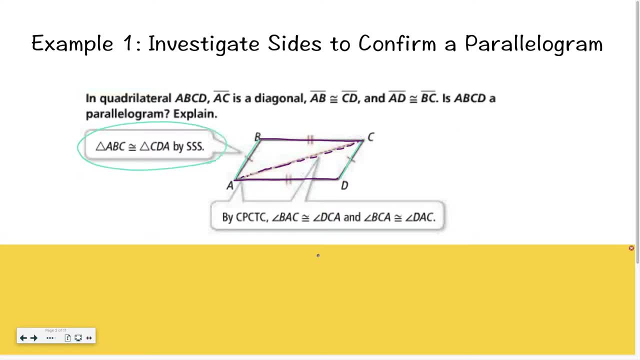 So a triangle ABC is congruent to triangle CDA by side-to-side. And you may be asking: why are we proving that the two triangles are congruent if we're trying to prove that it's a parallelogram? Well, the reason we do that is if we know that those two triangles are congruent. that means that we also have some angles. 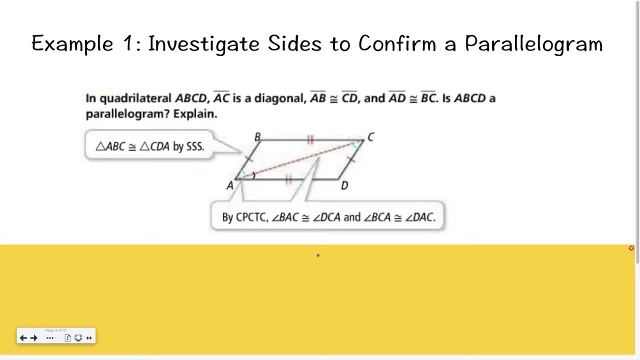 that are congruent and angles are going to play a big role in proving parallelograms. okay, So we know by CPCTC it's been a while since we've really thought about that. So that's the corresponding parts, so the parts that line up with each other. on, 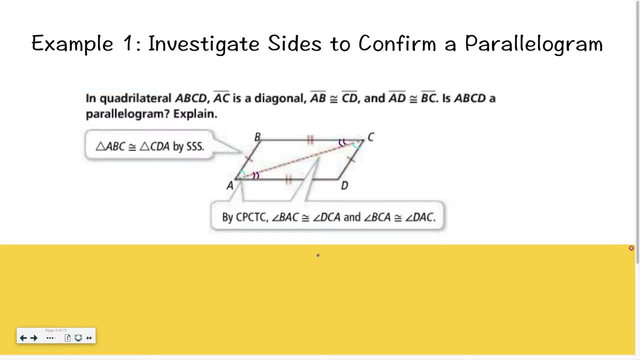 congruent triangles. so we already have those two congruent triangles are congruent. So I can say that those two purple angles are congruent to the two blue angles. and the reason that's important is if I know that those two angles are congruent, if I look at how they're related, 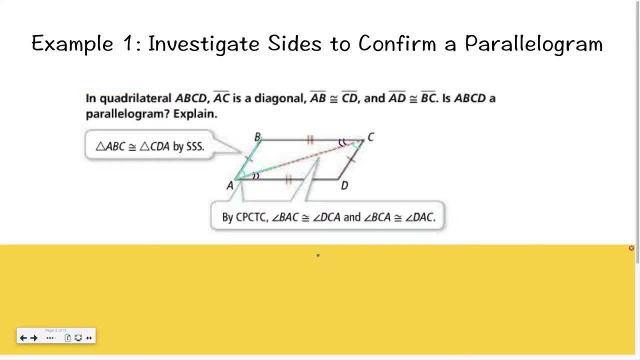 the blue angles. if I outline their shape, you can see we have two lines with a transversal cutting through and if we look at how these angles are related, we would say that they're alternate interior angles. They're between the parallel lines but on different sides of the transversal. 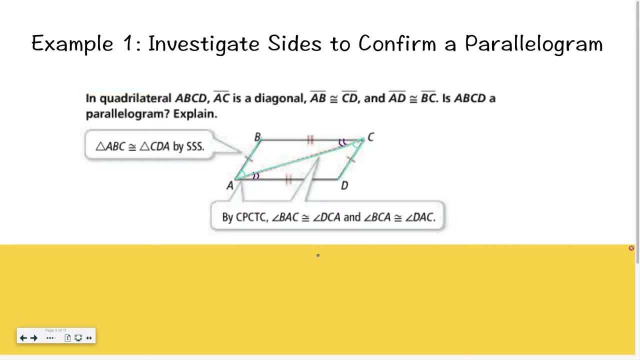 So, using the converse of alternate interior angles, I can say that segment AB is parallel to segment CD. and then I can do the same thing. I can say that: oh look, I have these congruent angles, even though my outlining was terrible there. 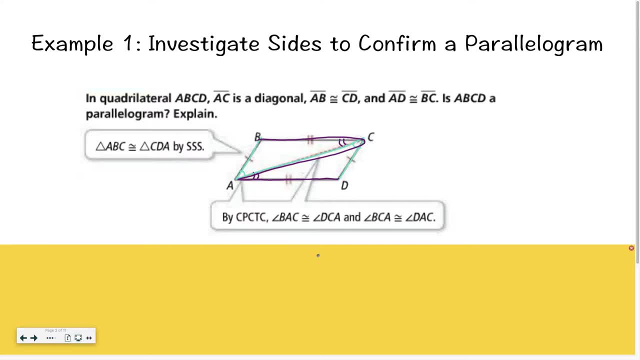 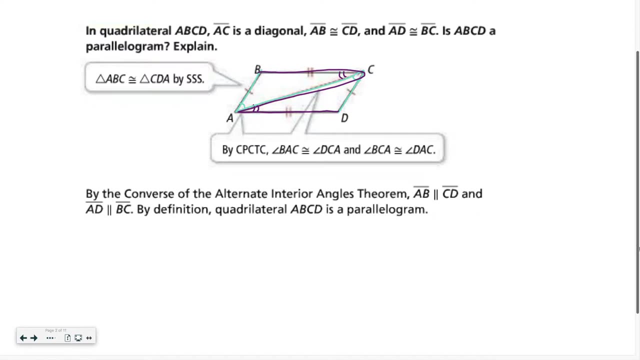 and that those are also alternate interior angles. So, using the converse again, I can say that segment AD is parallel to segment BC or C or CD and therefore, since I have two sets of parallel sides, ABCD is a parallelogram. 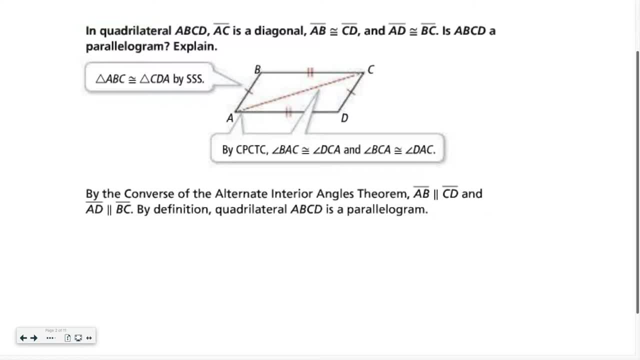 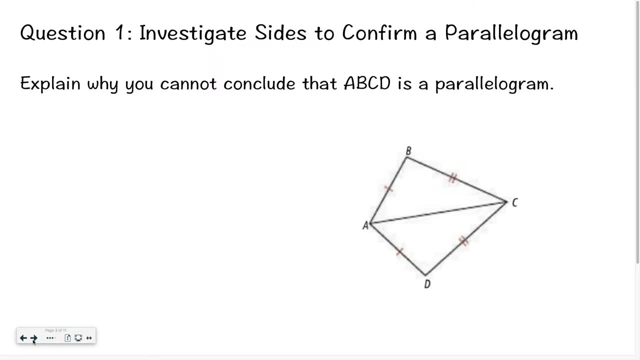 Okay. so you're gonna be using both angles and sides and sometimes breaking things up into triangles in order to prove that they are a parallelogram. So why don't you guys take a look at question number one and explain why you cannot conclude that ABCD is a parallelogram? Good luck. 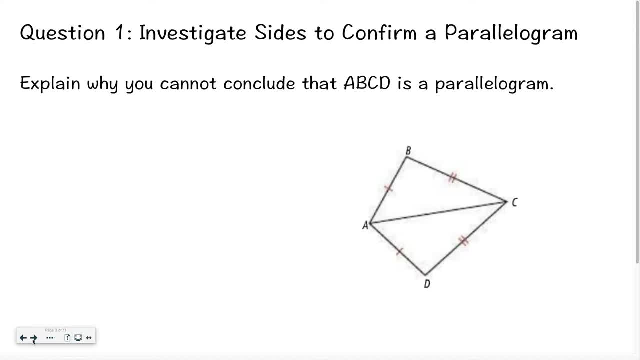 Hopefully you looked at this shape and you said something along the lines we talked about this yesterday: how, in order to be a parallelogram, you need to have opposite sides of a parallelogram. so the sides that don't touch each other are the ones that need to be congruent. but if you look at this figure, you'll see that the sides that are congruent are actually the ones that are touching each other, the adjacent sides. 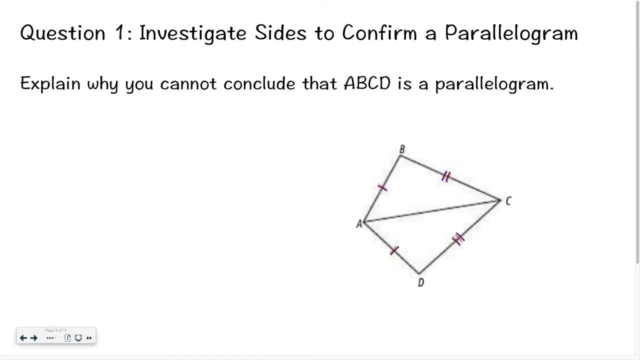 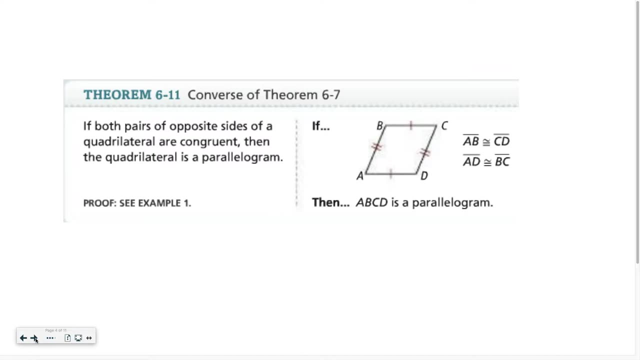 So you cannot conclude that ABCD is a parallelogram because it doesn't have opposite sides that are congruent. Alright, so then here is the theorem for that: If both pairs of opposite sides of a quadrilateral are congruent, then the quadrilateral is a parallelogram. 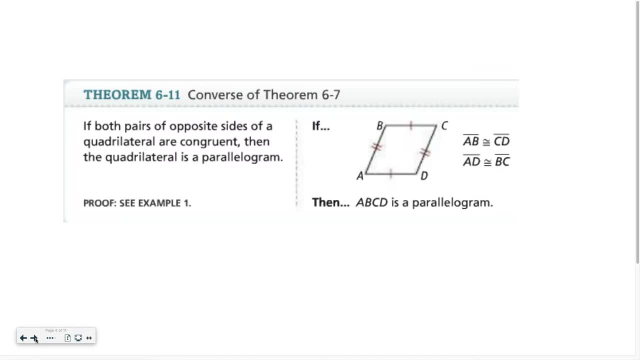 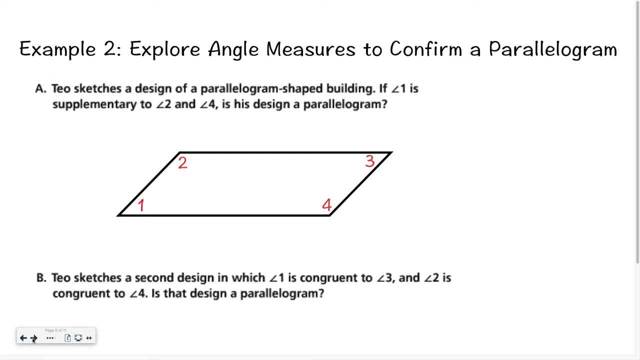 Go ahead and take a screenshot of that and add it to your collection. And let's start example two. So we have Teo sketches the design of a parallelogram-shaped building. If angle 1 is supplementary to angle 2 and angle 4, is his design a parallelogram? 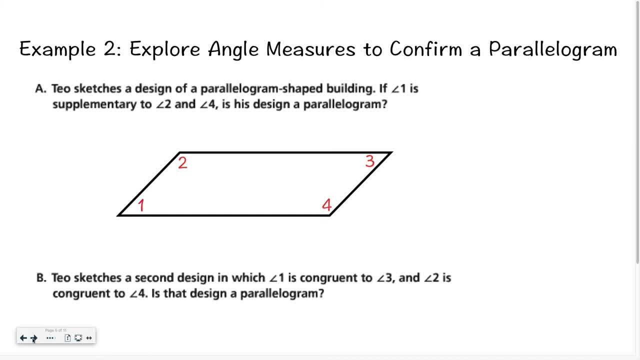 So if angle 1 plus angle 2 equals 180, because supplementary- remember supplementary- means 180, and we say that angle 1 and angle 4,, when added together, also equals 180.. Can we say that his figure is a parallelogram? 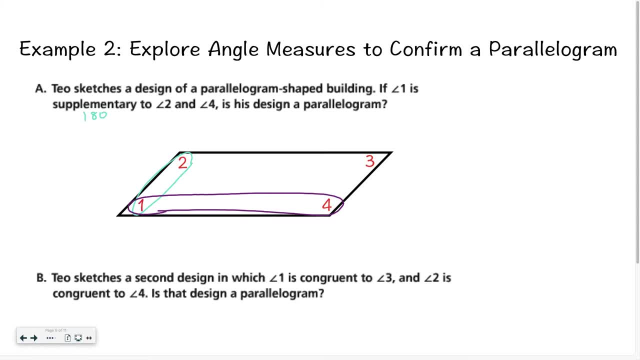 The answer is yes, And the reason being: if I look at how angle 1 and angle 2 are related and I think, okay, angle 1 and angle 2, I'm actually going to use a different color just to make it more apparent. 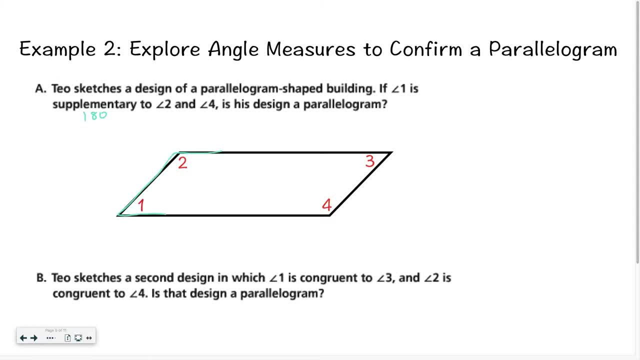 So angle 1 and angle 2.. How are they related? They are same-side interior angles. We learned about those way back when we learned all of our angle relationships. So same-side interior angles. we learned that if they are supplementary then their lines are parallel. 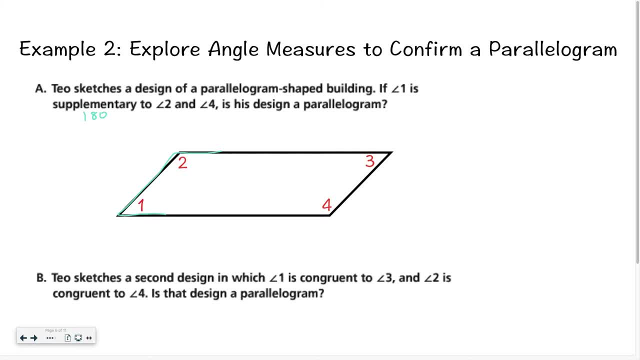 So since we know that angle 1 and angle 2 are supplementary, we can say the non-transversal line, So these two lines Are parallel. Then if I look and say, okay, now I have angle 1 and angle 4, and I know that those are also supplementary, I know that my non-transversal lines. so if I erase my transversal, my non-transversal lines are also parallel. 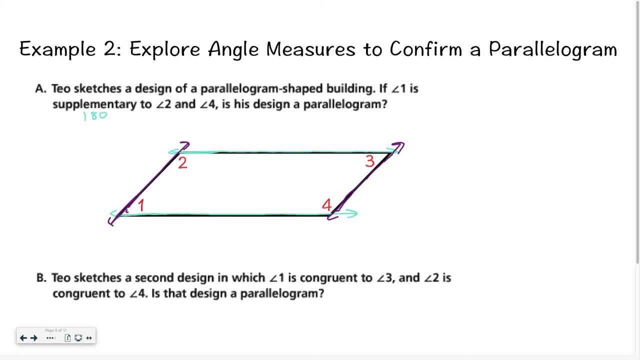 So that means these purple lines Are parallel. Now, if I look, I have two pairs of parallel sides. That means that this figure is a parallelogram. Okay, Now if we look at example 2, we have Tao sketches, a second design. 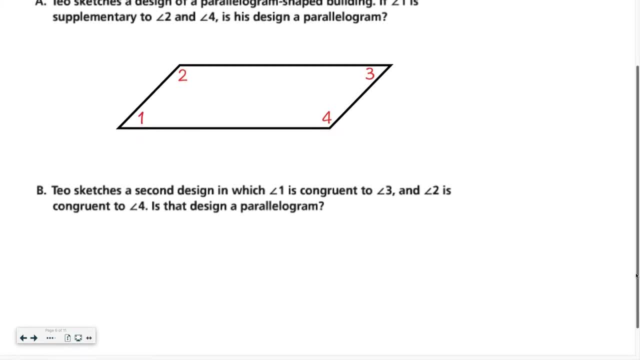 The second design in the book was pretty much the same design as the first, So I'm just going to use that same. So Tao sketches a second design in which angle 1 is congruent to angle 3.. So I know angle 1 and angle 3 are congruent and angle 2 is congruent to angle 4.. 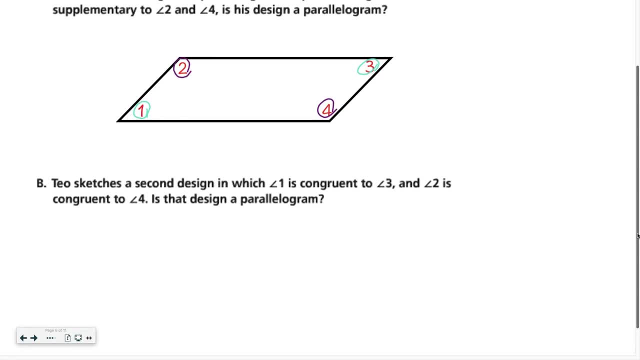 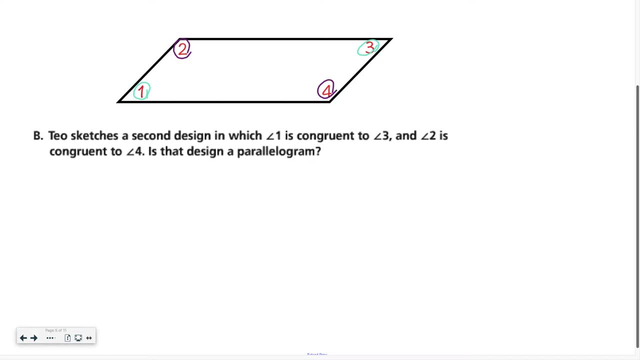 And I want to figure out: is that enough information to prove that it's a parallelogram? So if I think about it, I have four angles in a four-sided figure. So if I add all of them up, that means that they. 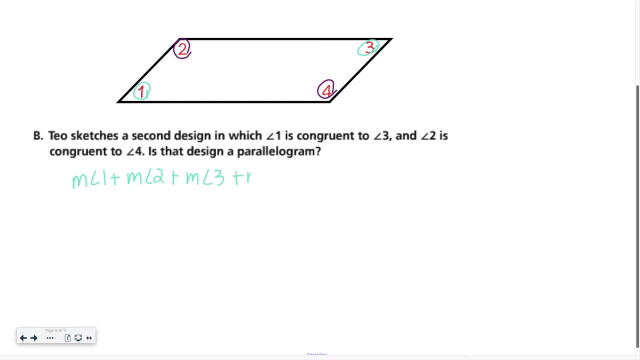 They should have a sum of 360 degrees. Now I know that the measure of angle 1 is congruent to the measure of angle 3.. So instead of writing measure of angle 3, I'm going to write measure of angle 1 again. 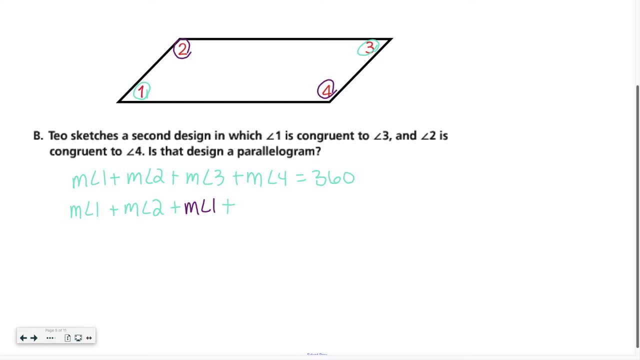 And then I know that the measure of angle 2 is congruent to the measure of angle 4.. So instead of writing measure of angle 4, I'm going to replace it with the measure of angle 2.. And now, if I look, I have 2 measure of angle 1 plus the measure of angle 2 equals 360, right? 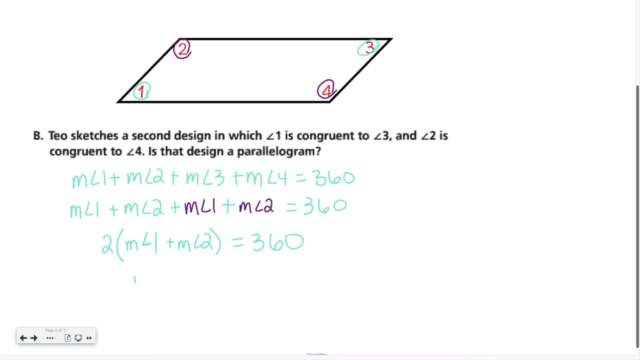 Because I can combine my like terms. If I divide both sides by 2, I have measure of angle 1 plus measure of angle 2 equals 180.. That means that they are supplementary And if I look at my picture, angle 1 and angle 2 are still same side interior angles. 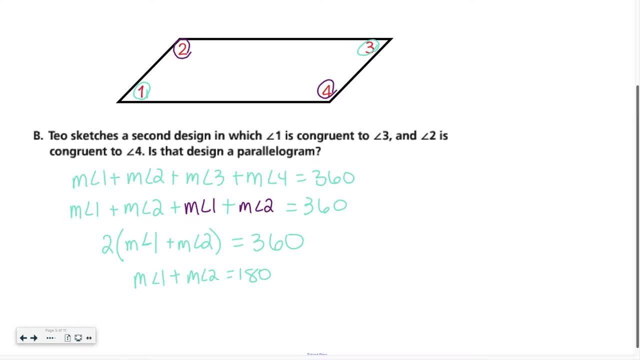 And if the same side interior angles are supplementary, that means their lines are parallel. So that means I have one set of parallel sides. And if I replace instead of saying measure of angle 2, remember measure of angle 2 equals the measure of angle 4.. 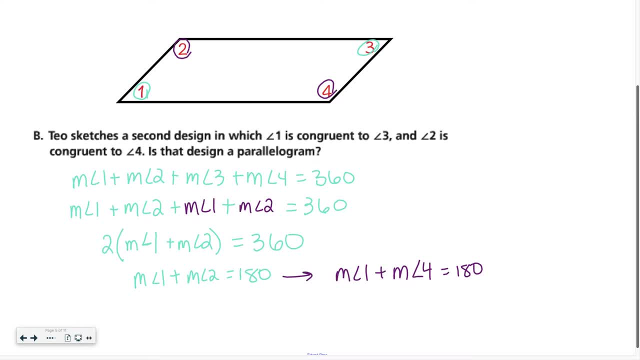 So I can substitute Measure of angle 4 back in. And now I know that angle 1 and angle 4, if I look at them, they are also same side interior And they're also supplementary. That means that their non-transversal lines are also parallel. 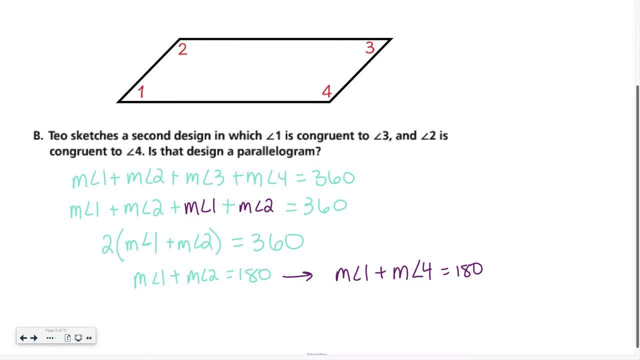 So now I have 2 sets of parallel sides, which means it is a parallelogram. What you need to have learned from this example is if you have angles that are congruent and, more specifically, opposite angles, meaning they don't touch each other. 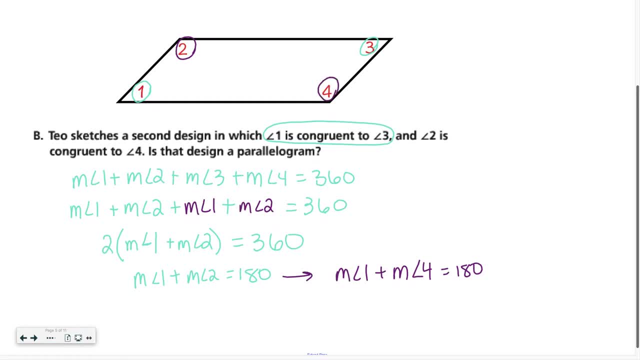 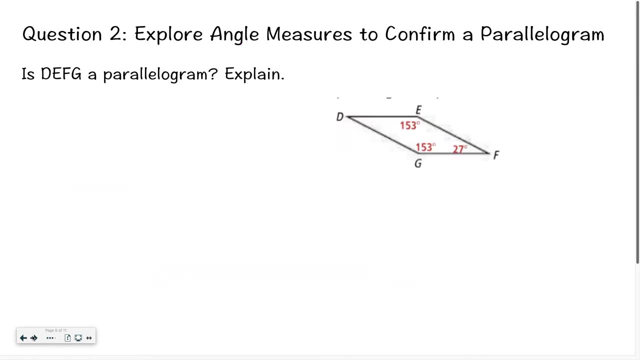 If your opposite angles are congruent, that means that the figure is a parallelogram. So if opposite angles are congruent, that means that the figure is a parallelogram. Why don't you go ahead and look at parallelogram DEF or figure DEFG and you're trying to state whether or not it is a parallelogram? 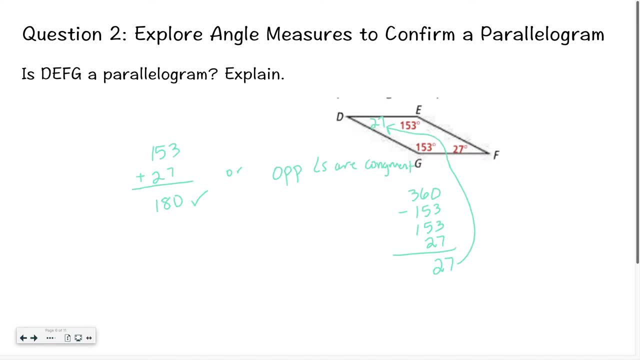 Good luck. Hopefully, for this example, you did either one of two things. You either said: 153 plus 27 equals 180, and therefore they are supplementary, And if they are supplementary, that means that if the consecutive angles are supplementary, that means that 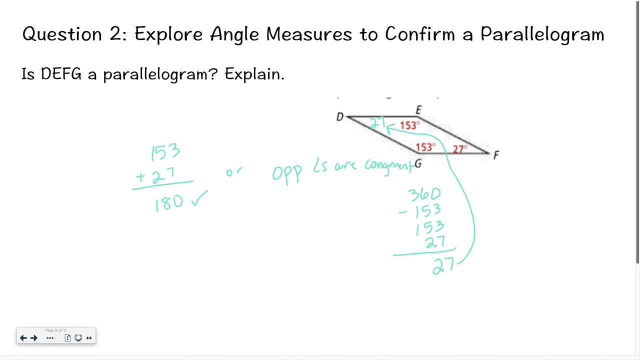 the figure is a parallelogram, which in this case they are, Or perhaps you said there's 360 degrees in there. If I solve for that last angle, it's 27.. And then my opposite angles are congruent, therefore making it a parallelogram. 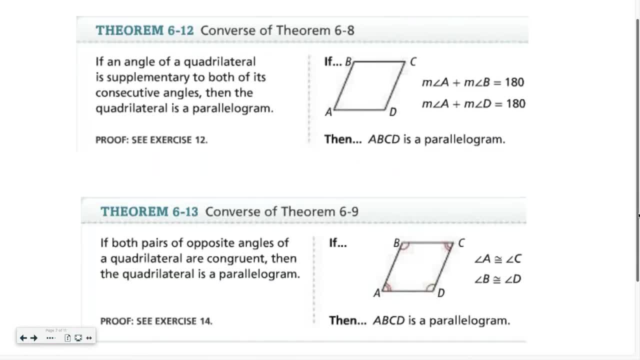 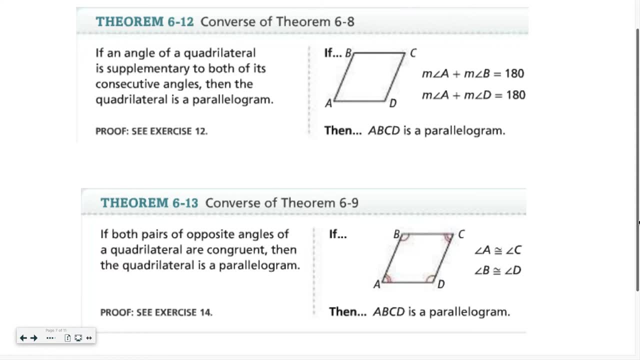 Both of those ways are totally acceptable. Here are two more theorems, So these summarize what we were just talking about. The top one talks about how if your same side angles are supplementary, it is a parallelogram. And 6-13 says: if opposite angles are congruent, then the figure is a parallelogram. 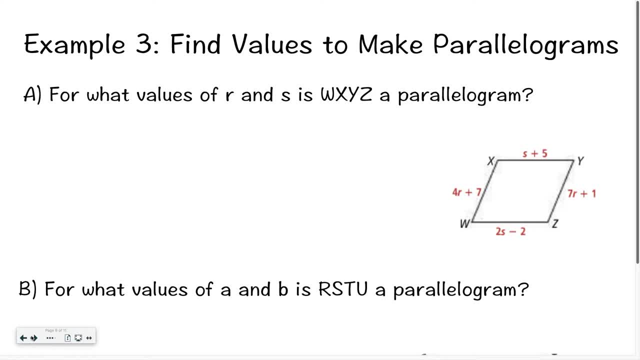 Alright. example 3. For what values of R and S is WXYZ a parallelogram? So if I know that I want a parallelogram and I know some facts about it, or that the opposite sides are congruent, 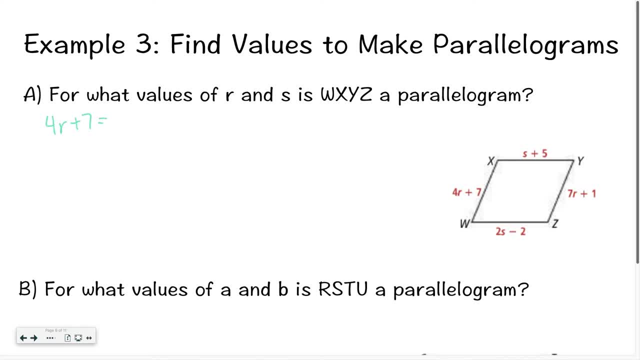 So that means I can say 4R plus 7 equals 7R plus 1.. And I can say that S plus 5 equals 2S minus 2. And solve from there. So if I subtract 4R from both sides, I have 7 equals 3R plus 1.. 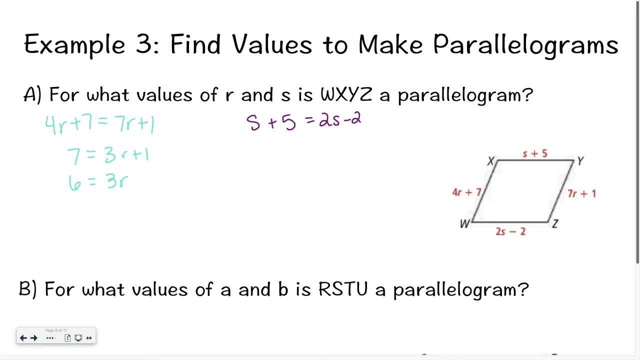 Subtract 1 from both sides, I get 6 equals 3R. Divide 3 on both sides and I get R equals 2, if my pen would work Then to solve for S. if I subtract S from both sides, I have 5 equals S minus 2.. 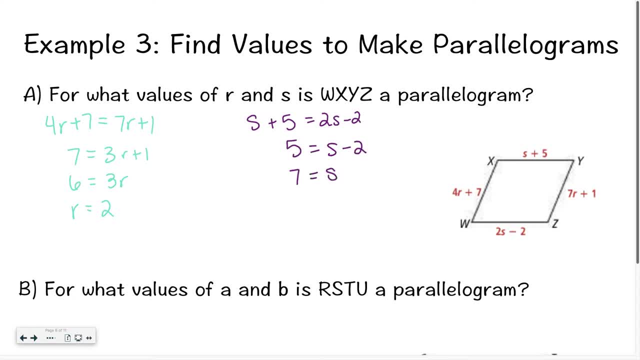 Add 2 to both sides, I get 7 equals S, S equals 7.. So if R equals 2 and S equals 7, that means this figure is a parallelogram, because its opposite sides will be congruent. 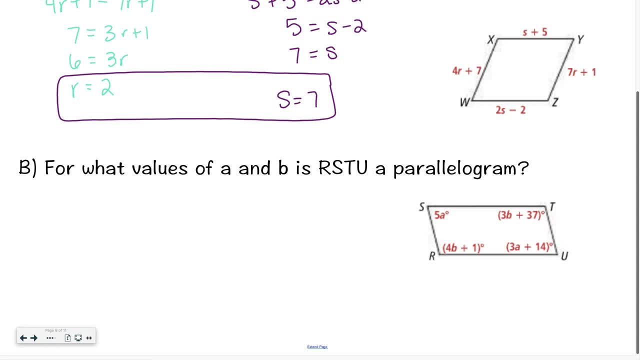 If I want to figure out if RSTU is a parallelogram, I have angles here. so that means my opposite angles have to be congruent. So if I say 5A equals 3A plus 14. Subtract 3A from both sides, I get 2A equals 14.. 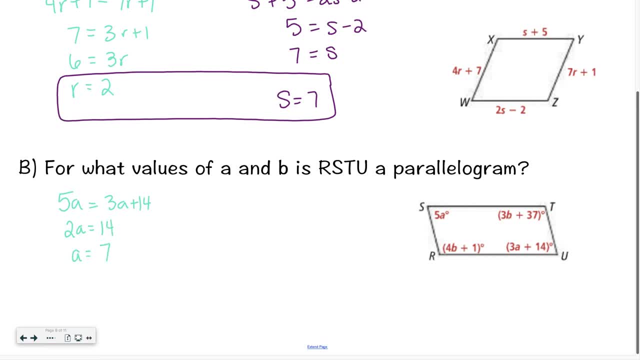 Divide both sides by 2, I get A equals 7.. And for the last set of opposite angles I say: 4B plus 1 equals 3B plus 37. Subtract 3B from both sides, then I'm left with B plus 1 equals 37. 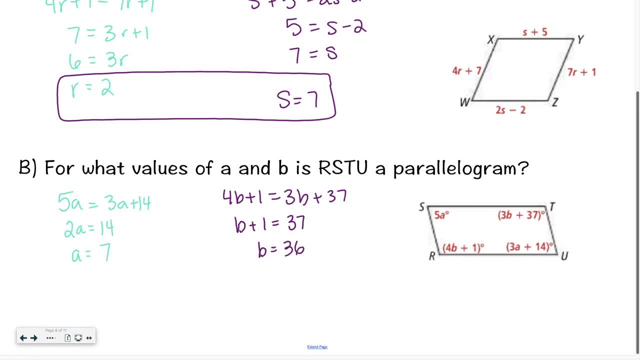 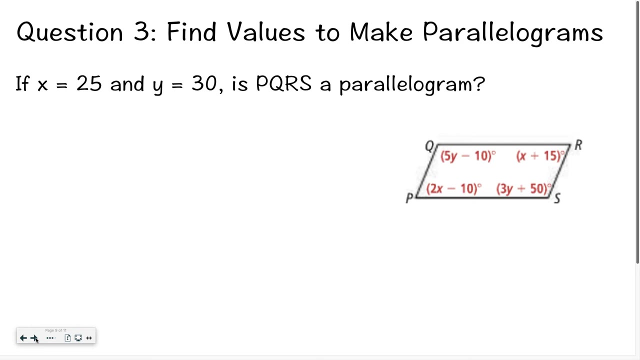 Subtract 1 from both sides and I get B equals 36.. So the second figure is a parallelogram: when A equals 7 and B equals 36.. Go ahead and figure out if X equals 25 and Y equals 30,. 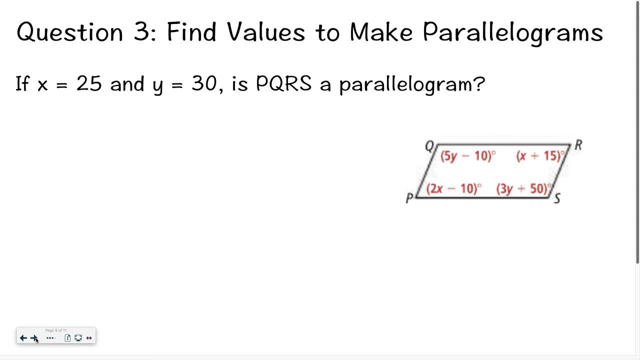 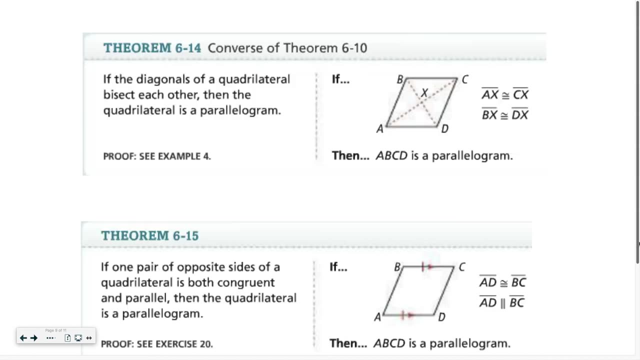 is PQRS a parallelogram a parallelogram? Good luck, Hopefully, for this question. when you plugged in 25 and 30, you found that those angles were congruent and therefore PQRS is a parallelogram. All right, and the last two theorems that summarize today's lesson are: 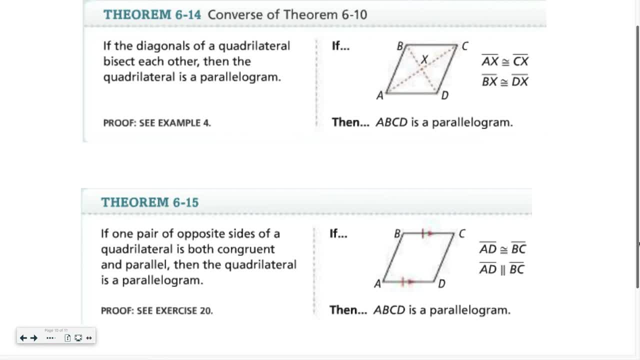 if the diagonals of a quadrilateral bisect each other, then the quadrilateral is a parallelogram. So if I gave you a parallelogram and I said ax equals xc or bx equals dx, that would mean that the figure is a parallelogram.